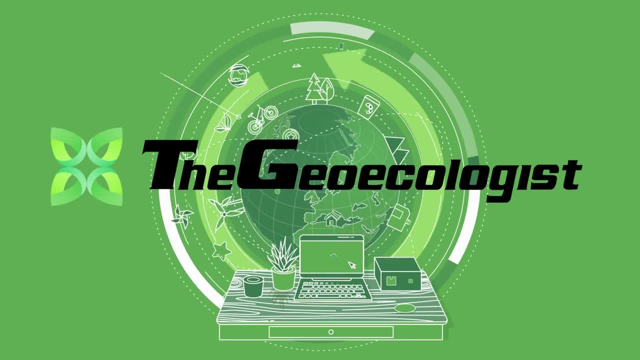 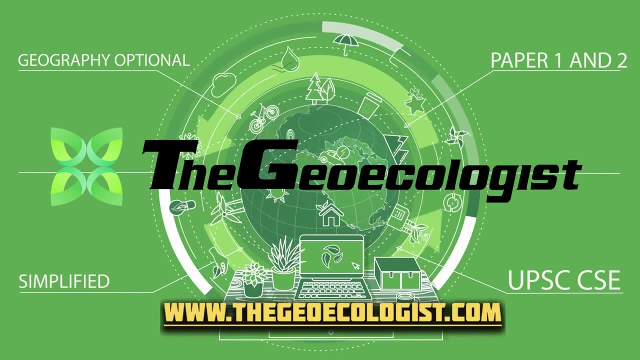 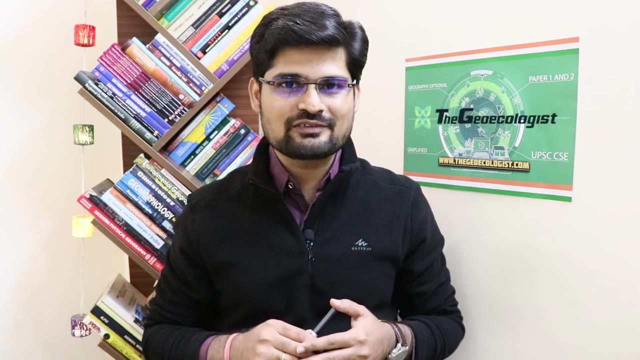 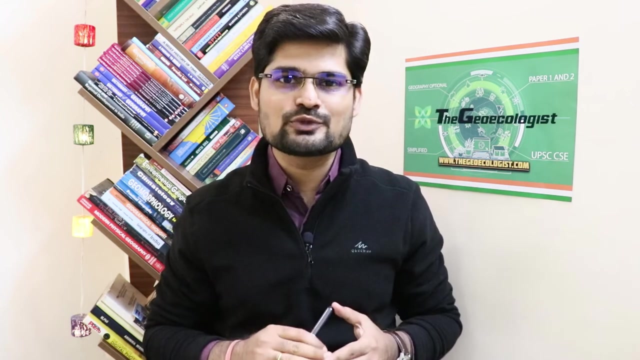 Hello everyone, Welcome to the Geoecologist. I am Dr Krishnanand and you have been watching my videos on oceanography and several other videos related to geography. In this session on oceanography, we are going to talk about the density distributions in the oceans, But 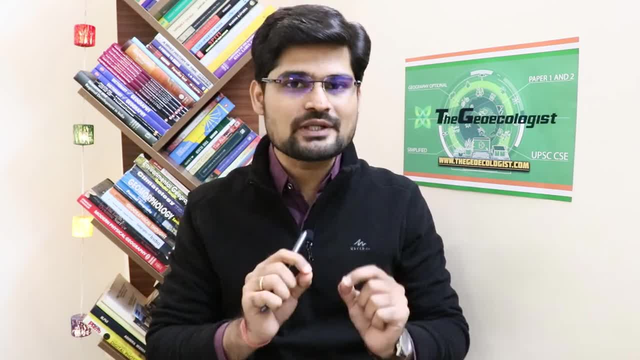 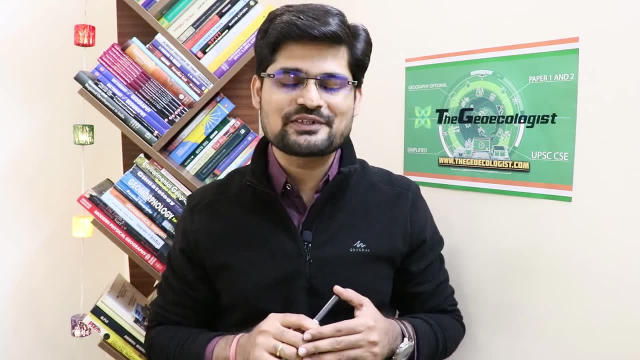 not just that, We are going to learn about the relationship of temperature density and salinity as well. So, before we go ahead, don't forget to subscribe to our channel and do share the videos with others as well. So now, after we have already learnt about the ocean's temperature distribution, 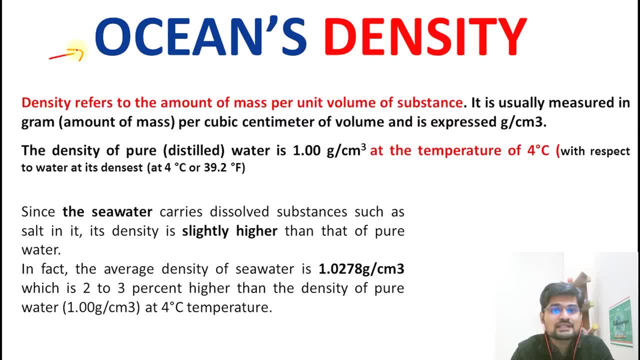 its factor. then we learnt about the ocean's salinity distribution and several factors. Today let's understand about the ocean's density distributions and factors associated with it. So density is what It refers to: the Amount of mass per unit volume. So remember, mass per unit volume is what we say is density. 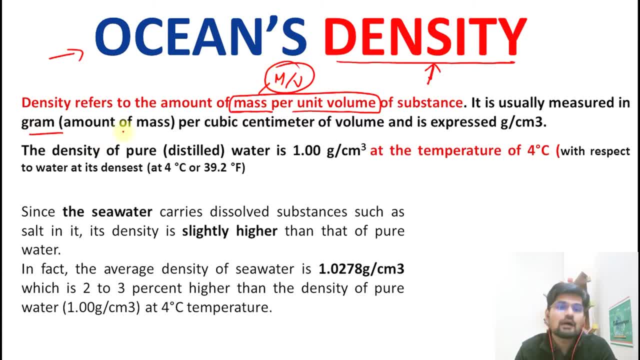 of a substance. So it is usually measured in what Gram amount of mass, that is, gram per cubic centimeter of volume, and is expressed as gram per cubic meter. So remember this is the unit. Now, when we are learning about ocean's density, the quantity is about water, So remember. 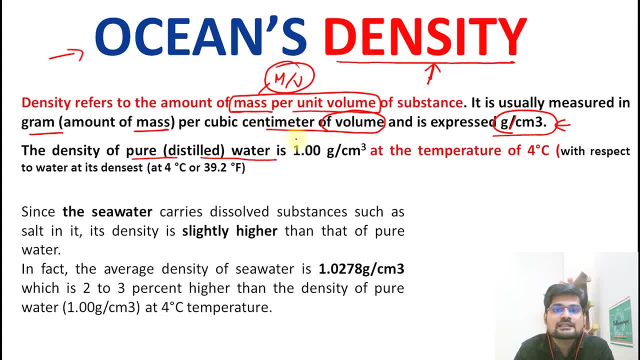 the density of pure or distilled water, we say, is exactly 1,, 1 gram per cubic centimeter, but at a given temperature, that is 4 degrees C. and why at 4 degrees C? because in comparison of the water at its densest, now remember, 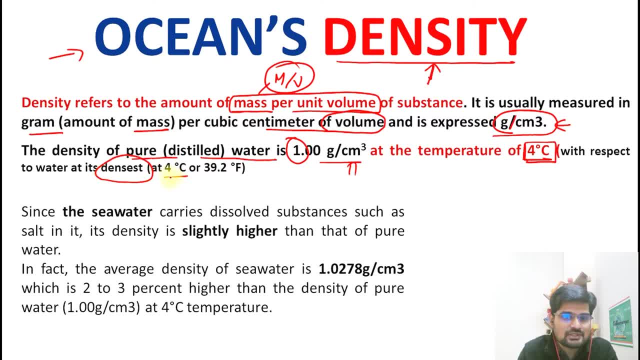 water is at its densest limit at this temperature. That is important to remember. That's why we take this temperature four degrees C for the comparison. So distilled water is 1 gram per cubic centimeter at four degrees C, And this is important to remember. Now, if we compare the distilled or the purest water to the salt, 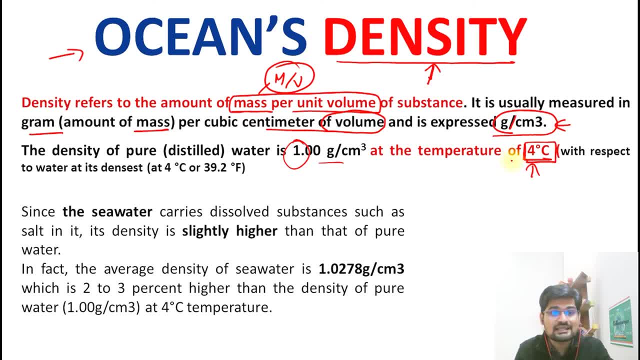 water. that is where we can understand how much more or how much less is there. So the sea water carries dissolved substances, as you know, and that is what we have already learned, in the salinity as well. that is the salt part, So its density is higher- obviously right- than the pure water. So 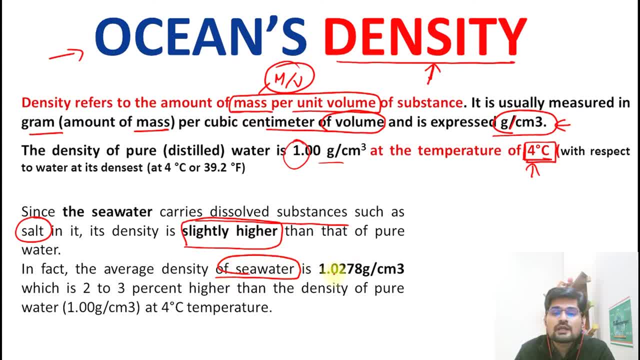 what happens? the average density of sea water is 1.0278 right, So 1.0278 gram per cubic centimeter, and this is what you say. is that from pure water it is increased, and how much? about 2 to 3 percent? 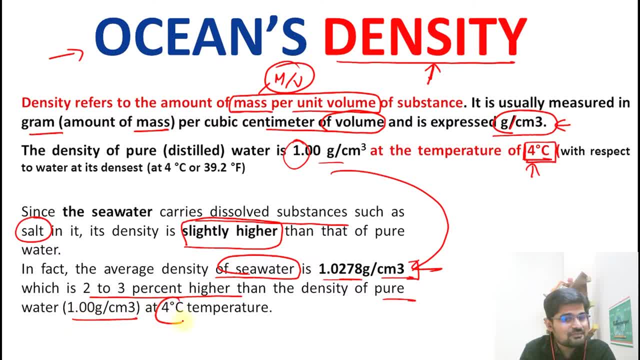 higher than the density of pure water at the same temperature, that is, 4 degree C temperature. So because of the density factor, and remember we are talking about the purity, So pure water is one value but 1.0278 as it goes. impure it means there are more dissolved substances. the density is increasing. 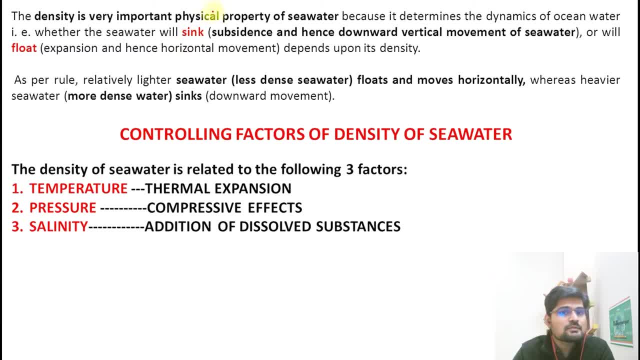 Now let's elaborate further more. So the density is very much important physical property of sea water and obviously because of the salt content, right so it becomes one of the most important physical property and we have learned in details in the salinity video as well, If you have not. 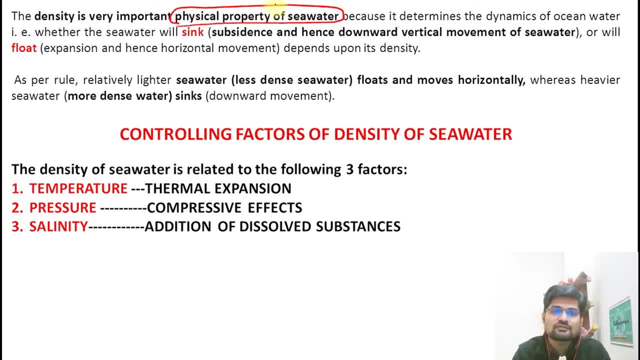 watched the video on ocean salinity. please go to the playlist of oceanography and do watch the video on salinity, where we have discussed in details the properties of saline water Right. so because of this, it determines the dynamics of the ocean water. Remember, dynamics is basically movement of ocean water: horizontal movement, vertical movement. 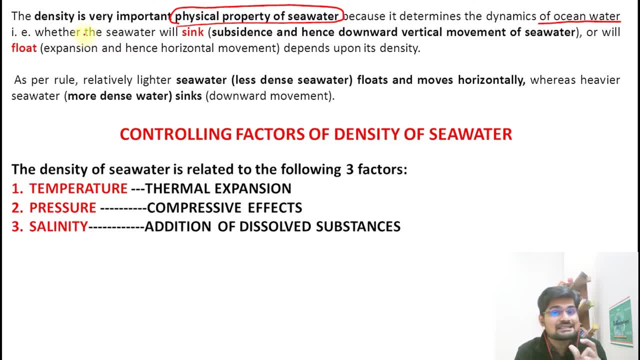 all these movement of water is triggered by this factor, that is, density factor, which is closely linked with the temperature as well as salinity factors. So what happens? seawater will sink. It basically means it will subside the subsidence process. It will go down and hence downward. a vertical movement of sea water will be triggered, right In one case. 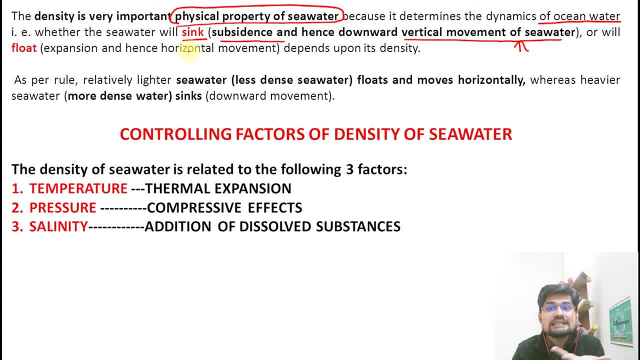 case, that is, when it is sinking, while if it is floating, if it is lighter, it is not heavier, it is less dense, then floating portion will be the expansion portion, right, So it will be expanding. it will be horizontal movement. So remember that density factor is linked to the 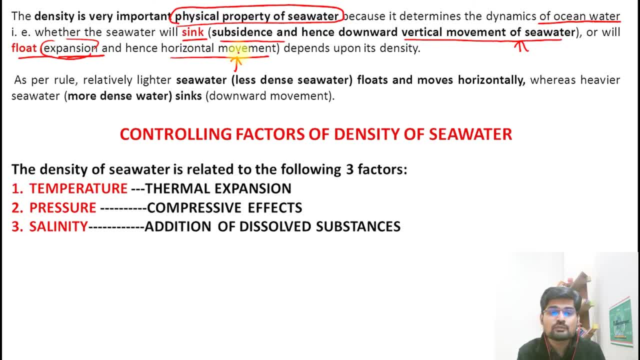 sinking or subsidence, as well as the floating and horizontal movement. That is why we term that density is one of the most important physical property of seawater that triggers or it determines the dynamics right. So, as per rule, the relatively lighter seawater. now, remember, relatively lighter. 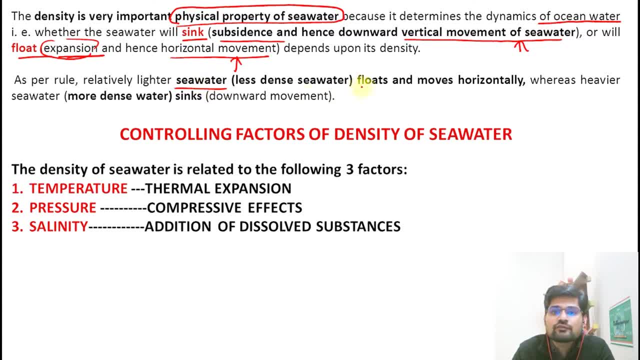 is less denser, that is what is lighter. So it floats and moves horizontally, whereas heavier water sits down or sinks down right. It triggers the vertical movement. So now, if you understand this, two important points: the controlling factors of density are these three factors. 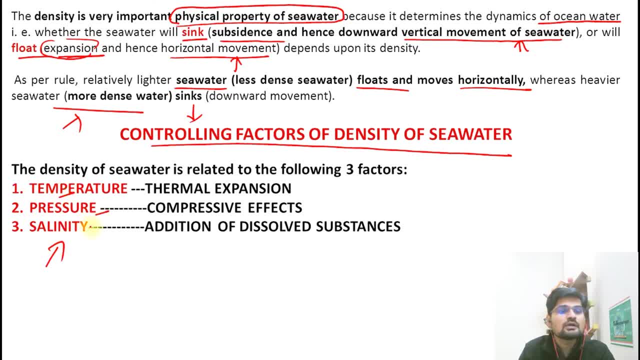 What are the controlling factors? One is temperature, one is pressure, one is salinity. So temperature, then we say it is about thermal expansion and contraction. If it is cool, it will contract. If it is hot, it will expand right. Similarly, pressure, if it is putting more pressure. 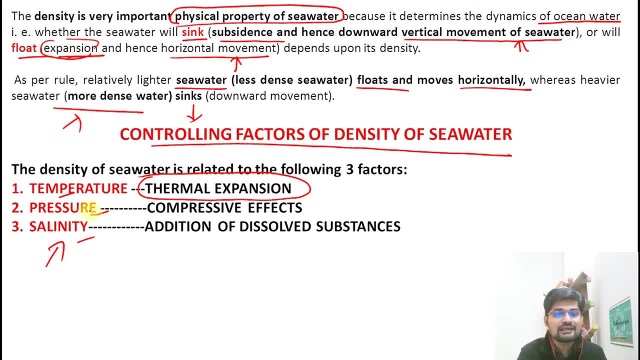 it is compressing it. If it is less pressure it is releasing it right. So that is important in terms of compression. And third factor we have already discussed in details: in salinity, that is addition of dissolved salt In a given amount of water. more salt it means, more dense it means 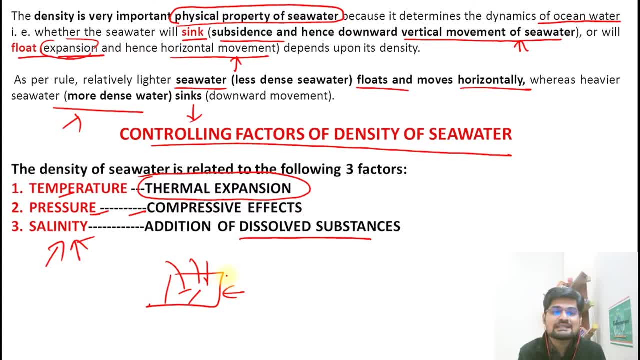 more heavy. it sits down right. So that is how salinity pressure temperature right. So this is how it is linked to the density of seawater. Now let us elaborate further more. So first important thing that we need to understand is the relationship. 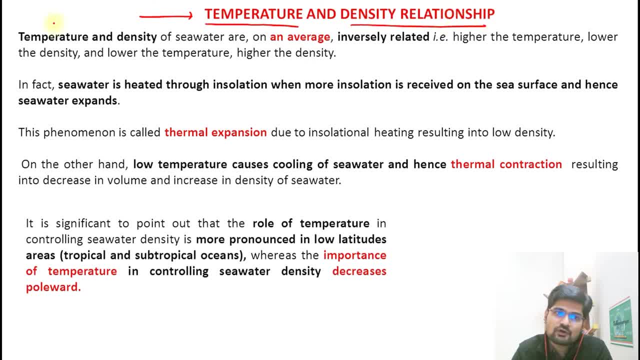 between temperature and density of the seawater. So temperature and density of seawater on an average are inversely linked. Remember there is an inverse relationship between temperature and density. So it means higher the temperature, lower the density. That is what inverse relationship. 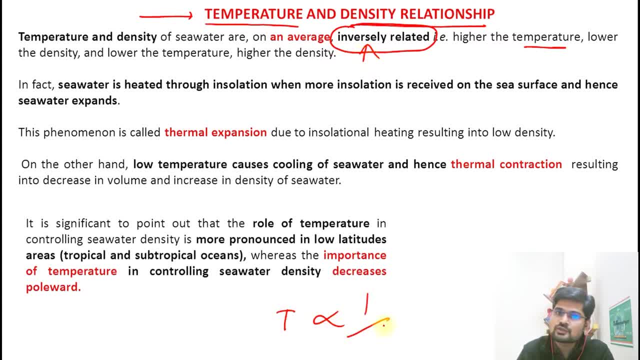 is. So remember T is inversely linked to the density of seawater, So it means higher. the density of seawater is inversely proportional to density, right In average condition, in normal condition, not in anomalous condition, because it is a dynamic phenomena, So there can be. 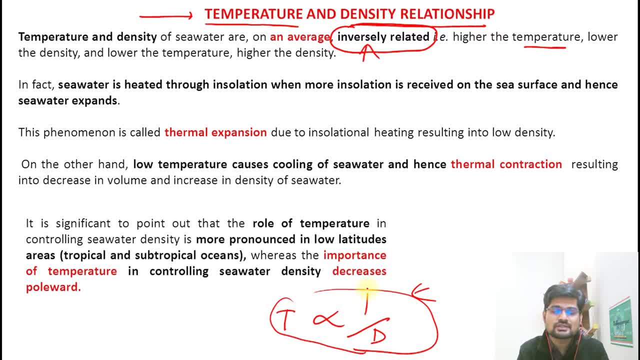 exceptions, But this is one. what we say is generalization. This is an average work that we understand, right So, lower the temperature, higher the density, right So, in this condition, what is important? Where is the higher temperature? Remember, in tropics it is higher. So what is? 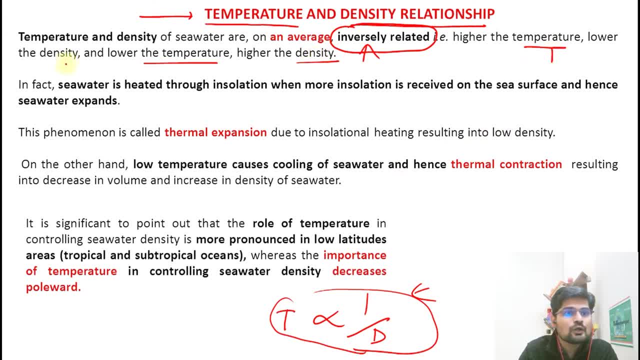 happening. The higher temperature is there and it is lower in density. So in this condition it is lower in density. That is why, if heat is there, expansion happens and movement of water is there, right. So what happens? Seawater is heated through insulation and when more 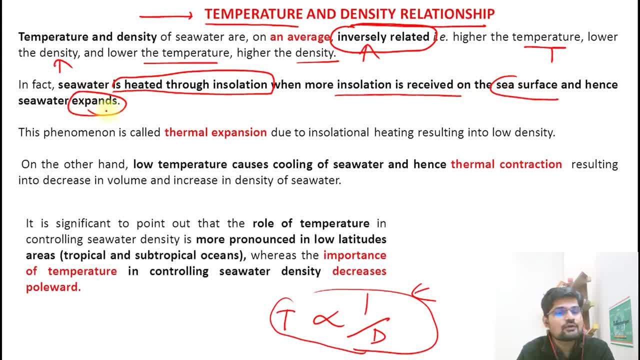 insulation is received, the sea surface expands right. Seawater expands because of temperature factor, So this is called thermal expansion, right, And remember what happens due to this: Density is now low there, right? Then, on the other hand, low temperature causes cooling. 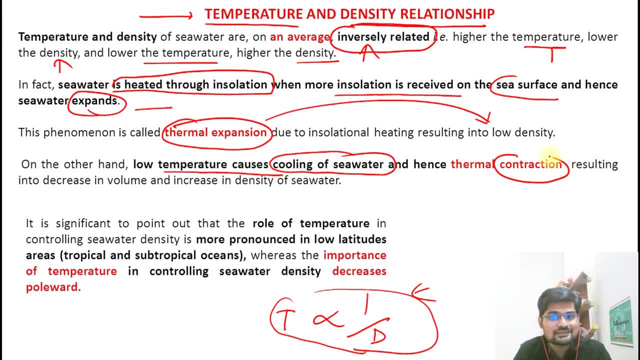 of seawater. right, And what happens? There is a contraction. So that is what thermal process is: Expansion, contraction resulting in the more density, more salts coming together, contracting. So that is what will happen here: The heavier or 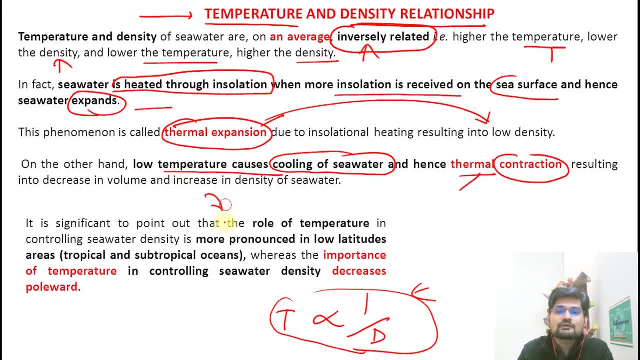 heaviness will increase. So it is significant to point out that role of temperature in controlling seawater density is more pronounced in lower latitudes and it is but obvious that maximum with tropical and subtropical seas which receive more insulation, obviously there will be lesser 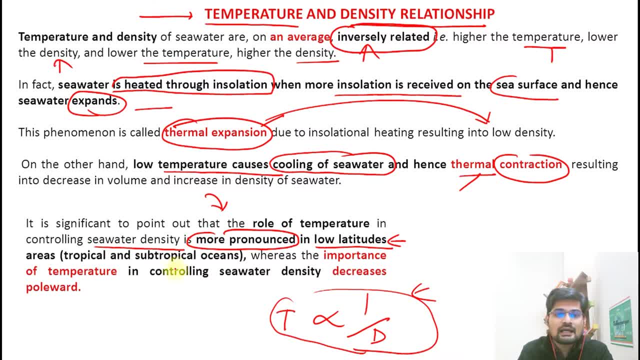 water, right. So temperature is important factor and remember importance of temperature in controlling seawater. density decreases towards pole volt. Remember as we go towards the pole, the temperature also reduces and its importance also reduces in terms of density right. So that is important point to remember in terms of relationship between temperature. 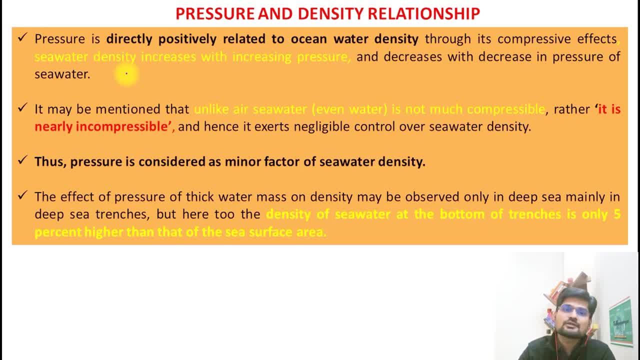 and density. Then let us talk about the second relationship, that is, pressure and density relationship. So it is directly positively correlated or proportional. It means pressure is directly proportional to the density. It means pressure increases, density increases, Pressure decreases, density decreases, right? So this is what 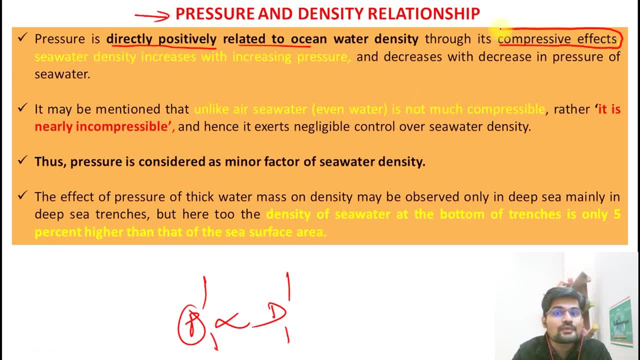 we say through compressive effect. Now remember, compression It means if this is mass of water and it is being pressed in, right, It means its molecules are coming closer to one other and that is where density will increase, right? So this is important here. So it may be. 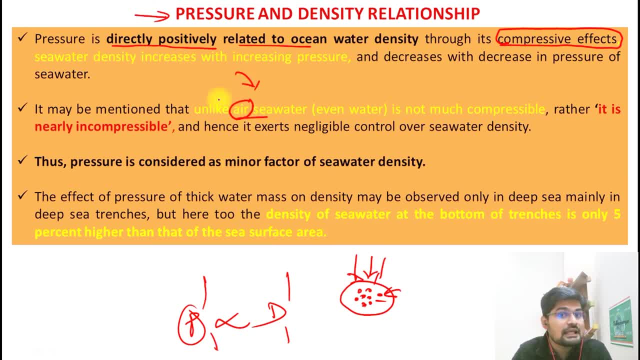 mentioned what, Unlike air, Remember, not like air, Seawater, even remember water is not much compressible. This is important to remember that water is not much compressible, It is not like air, Rather, it is nearly incompressible. 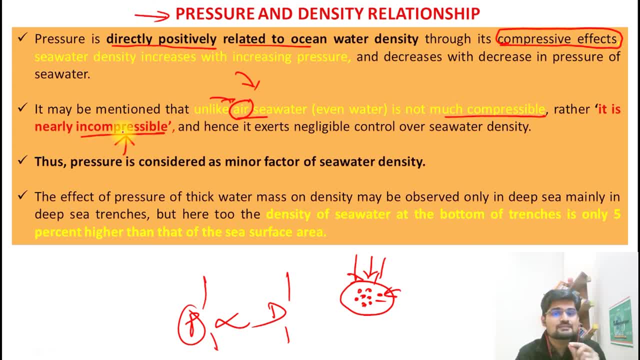 So almost compressibility factor is very less. That is important in terms of if we compare with the air. So do not get confused with the air pressure and water pressure relationship. Remember seawater is less compressible than air in comparison. 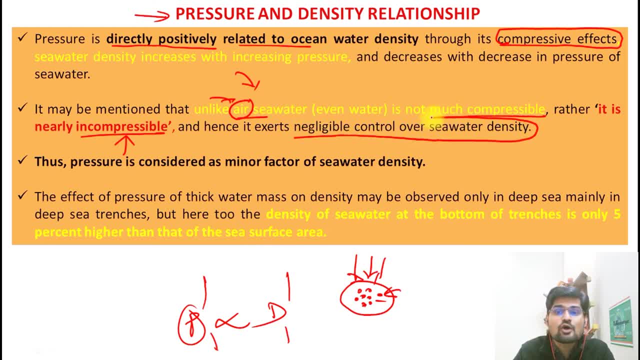 Hence it exerts negligible control over seawater density, Although there is a relationship between pressure and density, but this relationship is negligible. right, The pressure is considered as minor factor. This is important point to remember and when we want to study the example, 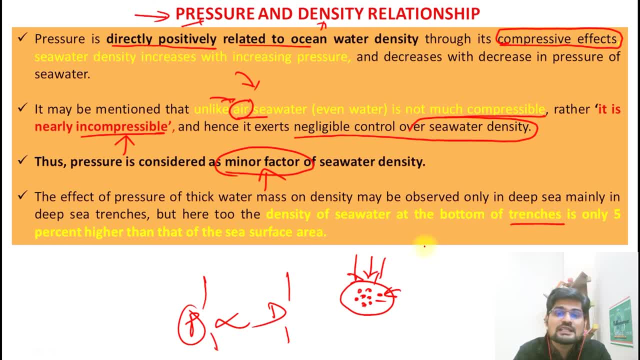 of this pressure. we can understand it through the trenches or deepest of sea bottoms, where there is 5% higher density than that on the sea surface. So just 5% of difference. right Pressure on sea surface is far lesser than that at a given depth. So this is just 5% change. 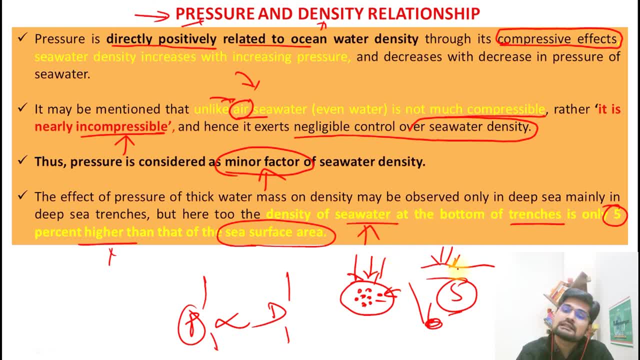 right In the deepest of trenches. if you observe, That is what it is supposed to be: a minor factor to remember. So pressure and density are positively correlated but pressure is just negligible factor or very minor factor in terms of the density control, but still it has a control. 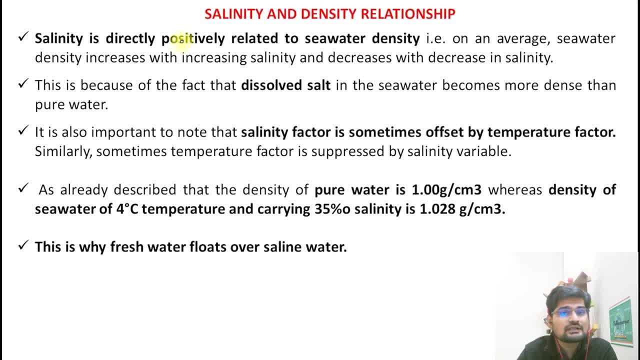 So that is a factor to remember. Then the third important point, which we have already discussed in the entire video. in the last video that was on salinity. So salinity and density relationship, Let us understand: salinity is directly, positively related to seawater density. So more saline. 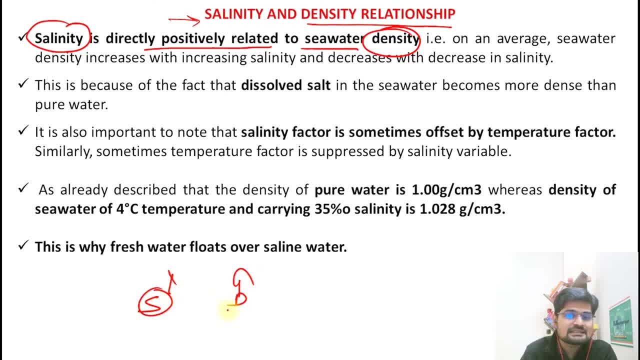 more dense. That is what we have learned, right? So salinity increases, density increases. Salinity decreases, density decreases, right, This is important. So this is because of the dissolved salt and remember, if this is a particular area, if there is a particular mass of water, 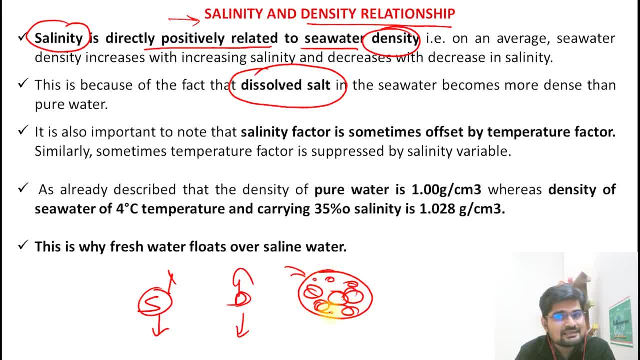 if there are more salts, it means that it is more dense, right? So that is the simple factor. It is also important to note here the salinity factor, sometimes offset by temperature factor. Now, temperature factor also, remember, is linked to the salinity factor, and that is why it will in turn change the density of that particular. 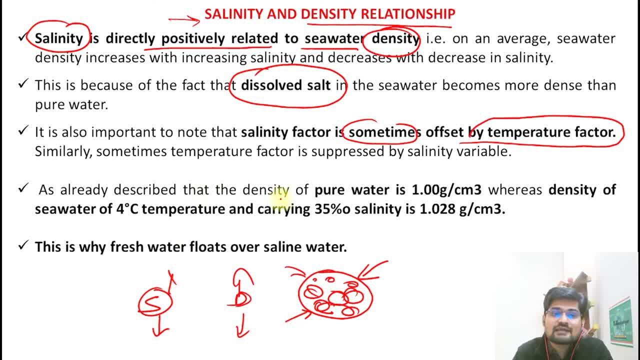 mass of water, right, So that is important. So, as already described, that density of pure water is 1, whereas density of seawater at 4 degree is 35, as we already know, right, And salinity is 1.028 gram per cubic centimeter, right? So remember, this is important, that. 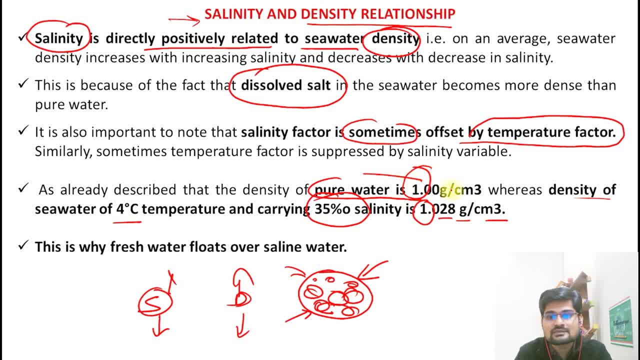 pure water, which is valuing here in terms of density, is 1 and saline water is. density is more Obviously, the salinity content is also 35 ppt right. So remember, salinity increases, density value is also increasing and that is why fresh water floats over saline water. This is 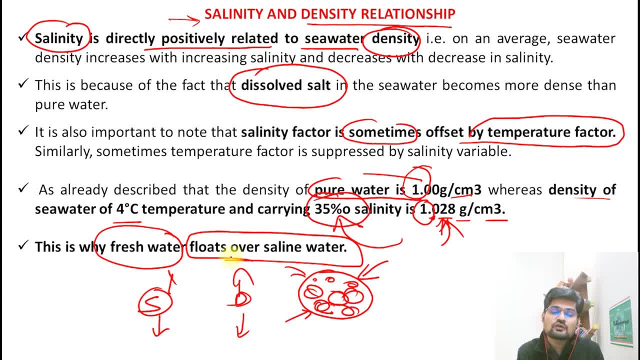 the relationship that we have studied, that fresh water will float over saline water because it is lighter, right, And also there is a role of temperature that we have already discussed in terms of density right. So this is how temperature, salinity, density are linked. 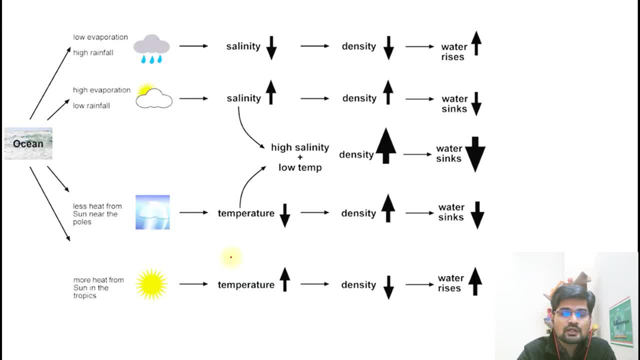 together, right? That is why it is important to remember. So if you want to draw a diagram for your answer writing, this is one diagram that I find fit. So if you see different cases first is lower evaporation, higher rainfall case. So what happens here? 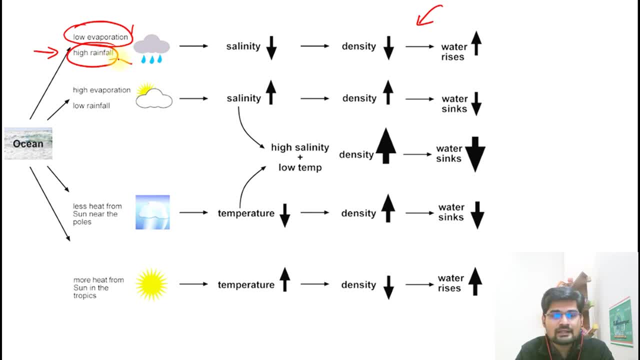 Here. evaporation is less, rainfall is more right. So what happens? Salinity will go down. Why? Because more water is being added to the system, So salinity will be lesser, So density will also be lesser, right? That is important to remember. Then, if there is higher evaporation case, 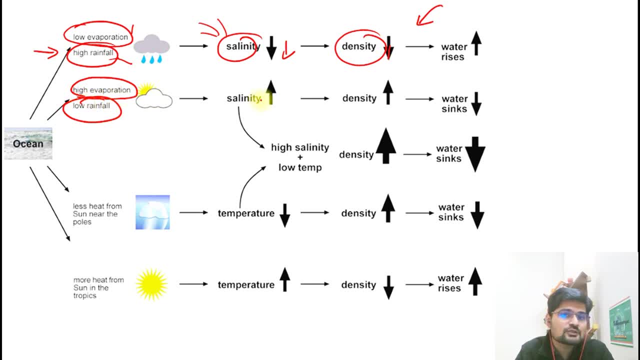 and lower rainfall case. obviously water is evaporating, So salt content is getting condensed in that particular place. It is concentrated, So salinity value will go up. It means density value will also go up and that is why the water will become heavy and water will sink down right. That is the first case. 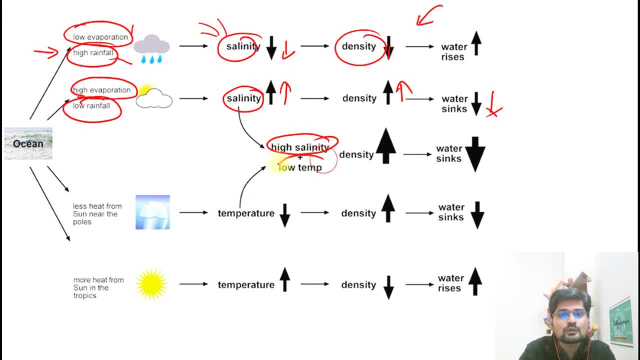 Now if you see high salinity plus low temperature, case right, density will automatically go up because salinity is high, temperature is low, So evaporation will be low and that is why heavy water it will sink down. right Now let us look this case: Less heat from. 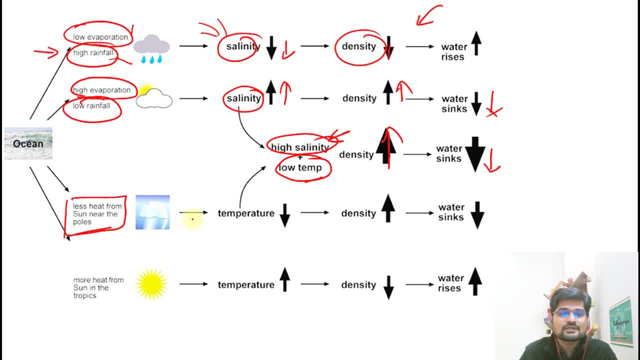 sun near the poles. So what happens? Obviously, temperature is less, and less temperature means less evaporation, right? So this is important. and density will be less, So less heat from the sun on the poles will be less. So what happens here? In this case, naturally, the challenge is that juddiness and the 그렇죠ness willгор on the poles. Okay, We will try to get rid of a problem. So the first request is: let us identify what the means of dissipation and—so let's discuss what is better. 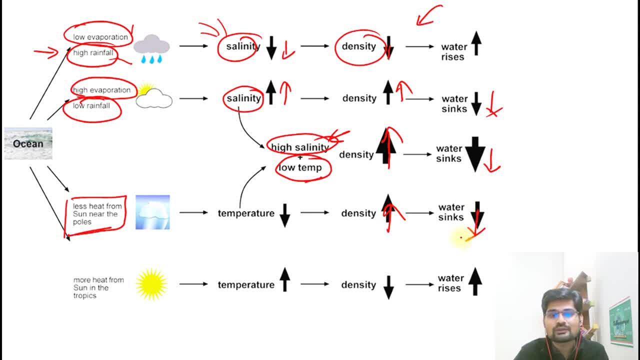 density will be higher and water will sink down. Similarly, in this case, more heat from the sun in tropics. it means what is there? More temperature is there. It means more evaporation is there. So density is actually going down because it is less dense. it is expanding. So what will happen? 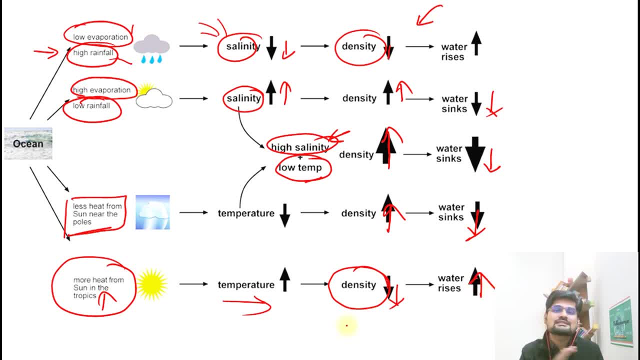 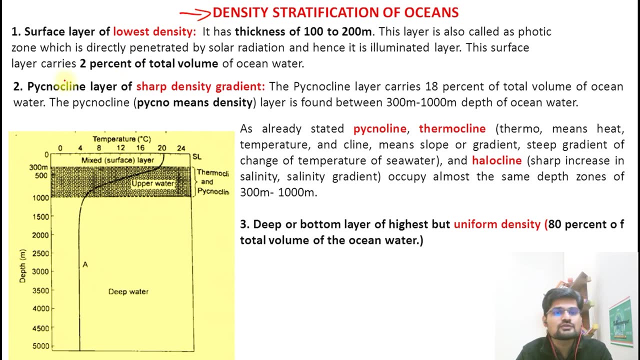 The water will rise. So this is how you can summarize it in one diagram. if you want to have the relationship of temperature, salinity and density That is important to remember here- Then if you want to stratify the oceans on the basis of density, you can stratify it into three. 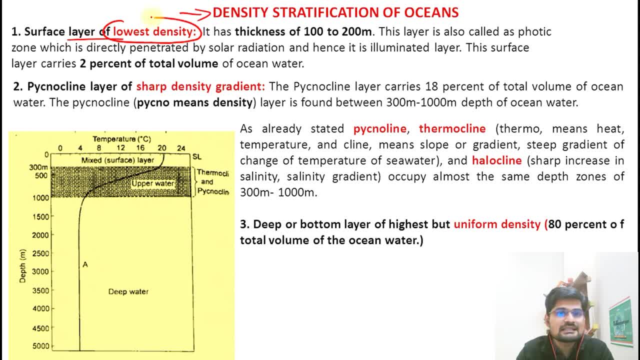 parts. That is surface layer that is lowest in density. lighter air is there in the upper part, So 100 to 200 meters thickness. It is called photic zone, Remember the photons. so light penetrating zone is there and it is about 2% of total volume of the ocean water. 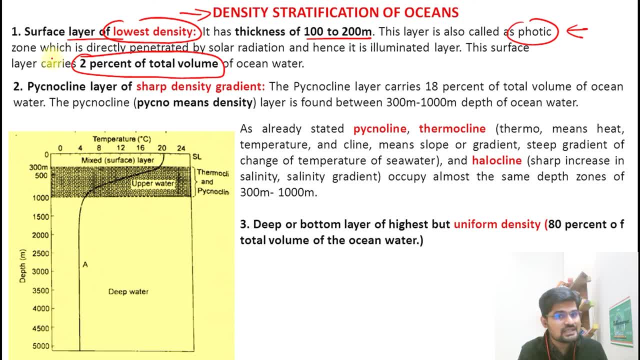 So this zone is illuminated, It has more phytoplankton, It is rich area, So it has less density, and less density also, remember, it is linked to less salinity. Then what we have is the pycnocline layer. The word pycno basically symbolizes. 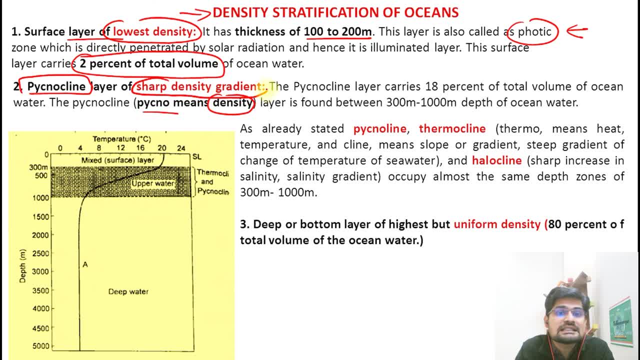 density. It means density, So it has sharp density gradient. Now remember thermocline and halocline. Similarly, you have the same layer where you have from this 300 to 1000.. This layer also is linked to what the temperature as well as your salinity factor. So that is where 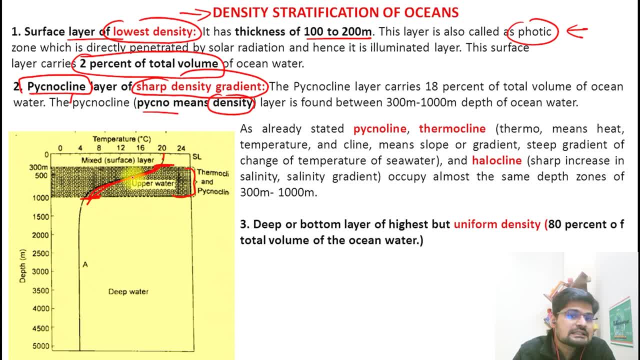 density is also linked. So this zone has sharp increase in density, if you observe right, Because this area, as you sit down it goes down right. Temperature is also less right And remember this is where pycnocline layer is there. So sharp density gradient, remember it is. 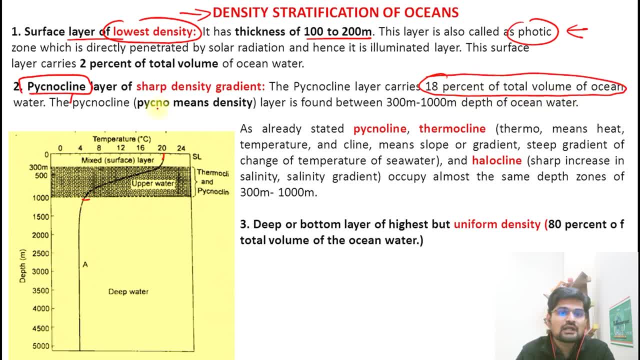 18% of total volume of ocean water and what happens in pycno, basically, is density change and, as already understood, that pycno-cline, thermocline, halocline, remember. thermo is the for heat, halo is for sharp decrease or increase in salinity. So picno, thermo halo, Remember. 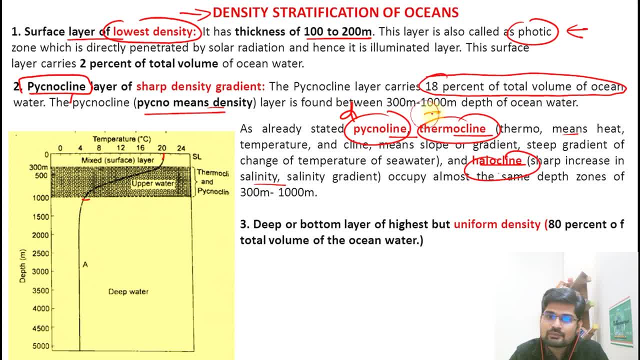 these are all linked to what? Density, then temperature and then salt, that is salinity. So picno, thermo and halocline is the same layer. that is 300 meters to 1000 meter where there is a sharp increase or decrease depending upon the situation. right So deep bottom area is the 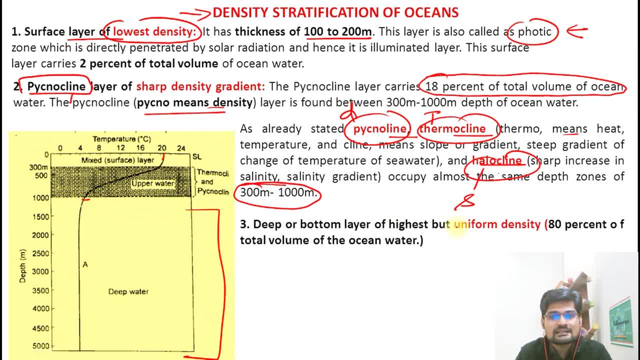 third portion, right In terms of stratification, and that is having a uniform density. Remember, 80% of the ocean total volume is there. Density is uniform, temperature is uniform, salinity is also largely uniform. So we have already learned about these relationships, right? So density, 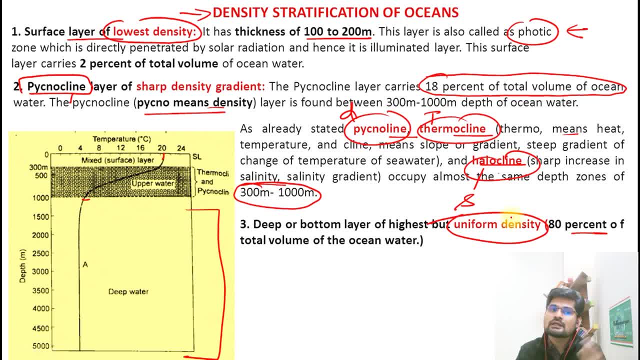 stratification of oceans is into three zones: The upper zone, the intermediate, that is the middle zone, or we can say transition zone, which is called picnocline, and then what we have is the deep or the bottom layer right. So that is the density stratification of.